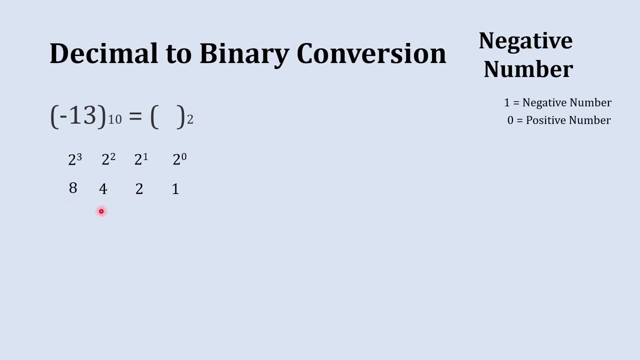 So, in order to convert this decimal into binary, we will add these numbers together. So first we will take this 8 and we will add this 4 into 8.. So it will become 12.. Now, if we add 2,, it will become 14.. 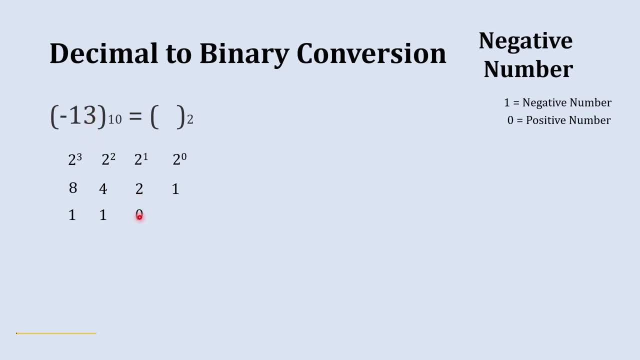 So our number is 13,, right, So we will take it 0.. So we will not add this 2.. Then again, we will add this: 1. So 8 plus 4, 12 plus 1, 13.. 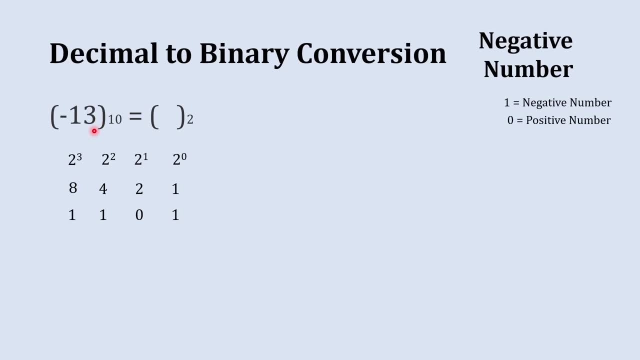 So this is the binary equivalent to positive 13.. Now, Now it's time to convert into negative. So whenever you want to convert it into negative binary number, there are two rules. The first is you're supposed to convert to first complement and then you're supposed to convert that into 2's complement. 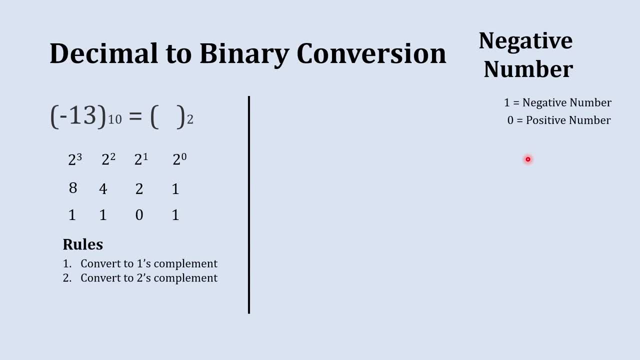 So let's do it over here. But before moving ahead, I would like to point out a very important thing, and that is: the representation of the number is in how many bits? Here the number is represented in 4 bits. You can represent number in 4-bit, 8-bit, 16-bit, 32-bit in this manner, right? 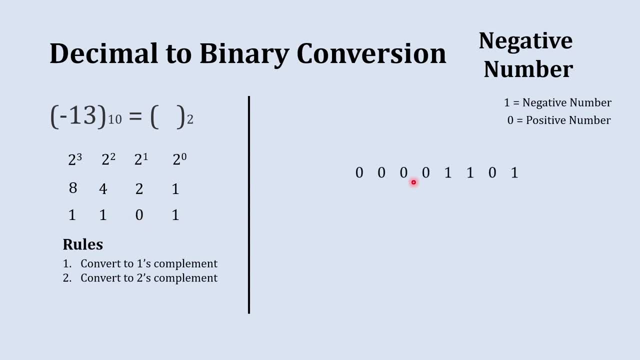 So here we are representing this number, the same number, in 8-bit manner. You can even solve it using only 4-bit manner, but why I'm taking 8-bit, that I'll tell you a little later. So the first step is to convert this into 1's complement. 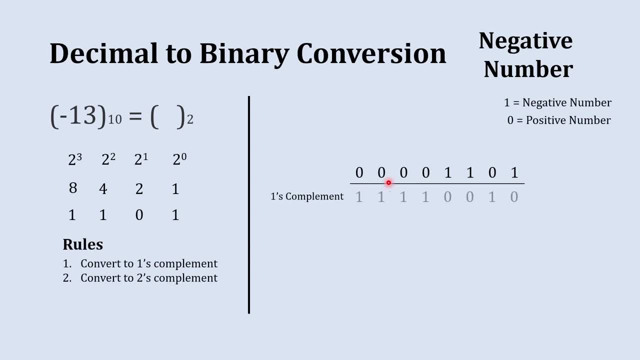 So when we want to take 1's complement, it's very simple: Whenever there is 0, write 1.. And whenever there is 0, write 1.. And whenever there is 1, write 0.. So this is the 1's complement of our number. 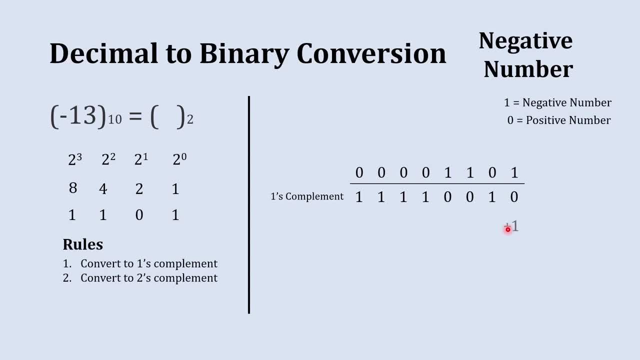 Now we'll go for 2's complement. In order to get 2's complement, we're supposed to add plus 1 into 1's complement, And whatever answer we'll get, that will become our 2's complement. So here we'll add plus 1 into this number. 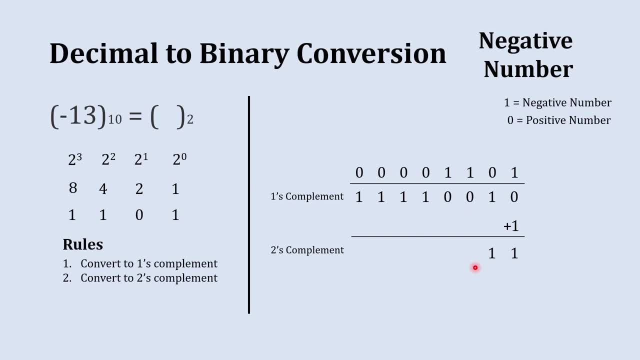 So it will become 1, this one as it is, and the remaining number will be as it is. So this is our 2's complement representation, And this number is binary equivalent to negative 13.. If you are using 4-bit representation, then you're supposed to write 0011.. 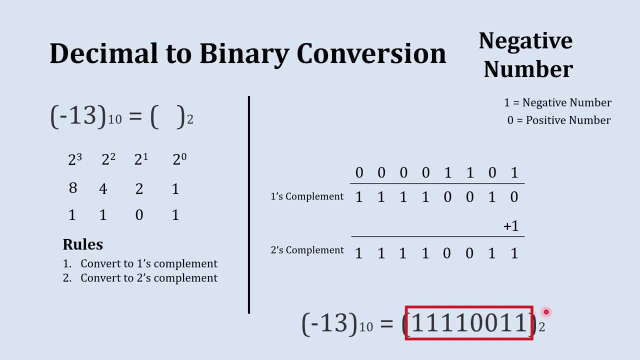 And if you are using 8-bit representation, you're supposed to write in this manner. Now you just dive into our animated playlist on number system, logic gates and more in digital electronics. It is specially designed for you, So get ready to explore the digital electronics. 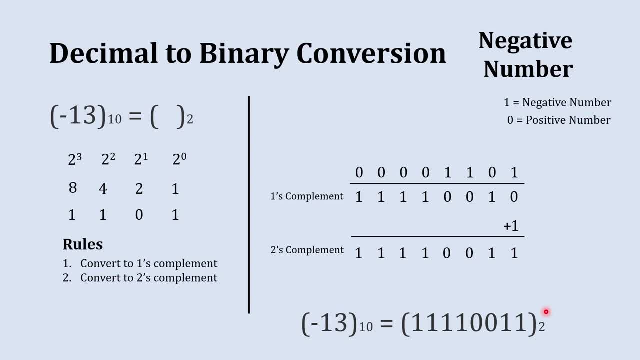 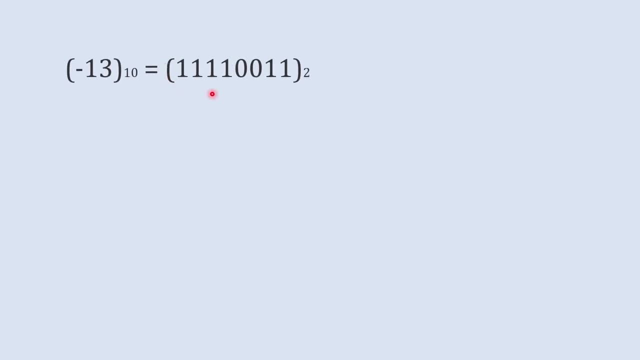 World and to explore that. the link is given in description and above here in I button. Now it's time to verify this answer, whether this answer is correct or not. So, in order to verify what we'll do, we'll take this number and we'll try to convert back it to decimal number. 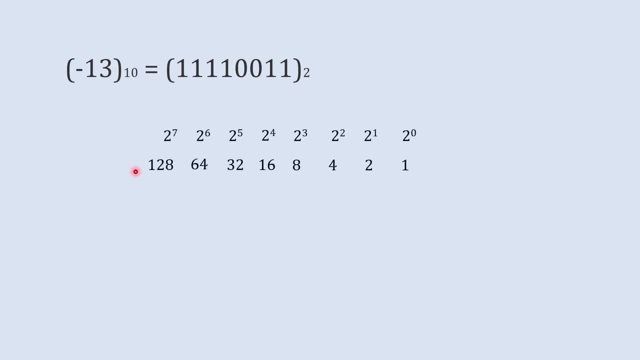 So let's convert this binary into decimal. So get ready with this decimal numbers And then multiply it with our number 11001111.. But now here, this is the minus 1.. Why it is minus 1? Because your most significant bit is 1, that represent it is a negative number. 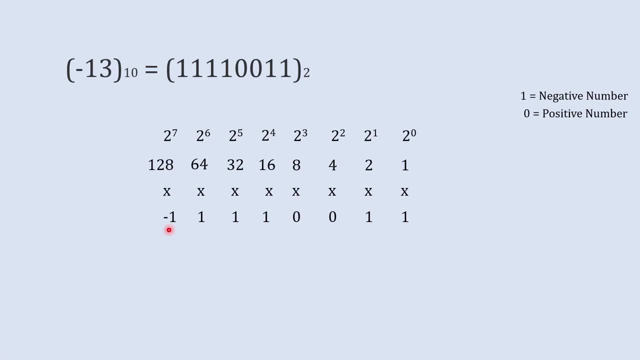 So here we are taking this as a minus 1. And why we supposed to do it? If you want to understand that thing in detail, I have explained all these things in my previous separate video, So you can watch that video to clarify this concept. 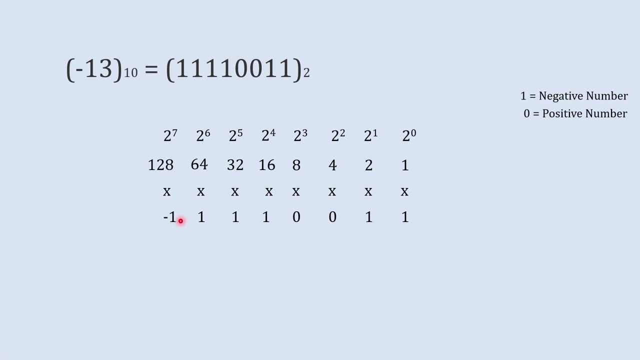 Except of taking minus 1.. So now we'll multiply this 128 with minus 1.. So it's minus 128, it's 64,, 32,, 16,, 0,, 0,, 2 and 1.. And now it's time to add all these things together. 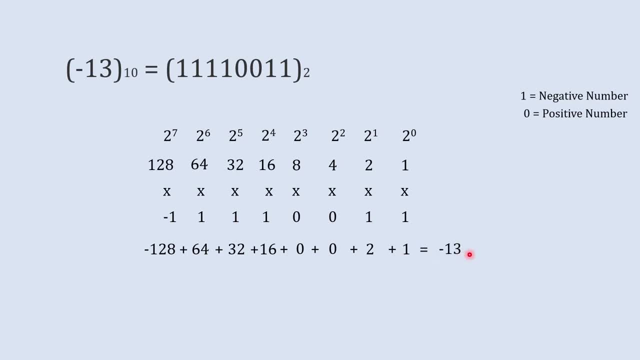 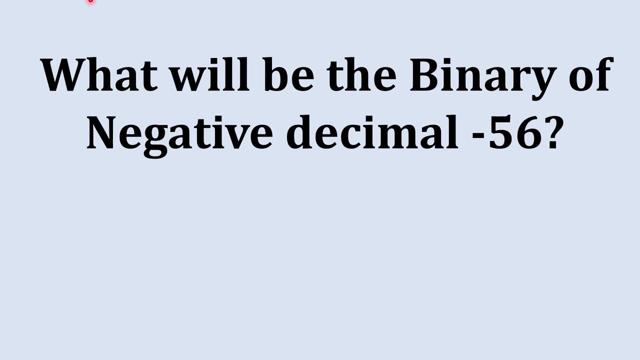 So when we add all these things together, we'll get minus 13.. So that is how we can say that this binary number is equivalent to minus 13.. Now pause for a moment and tell me What will be the binary of negative decimal minus 56?. 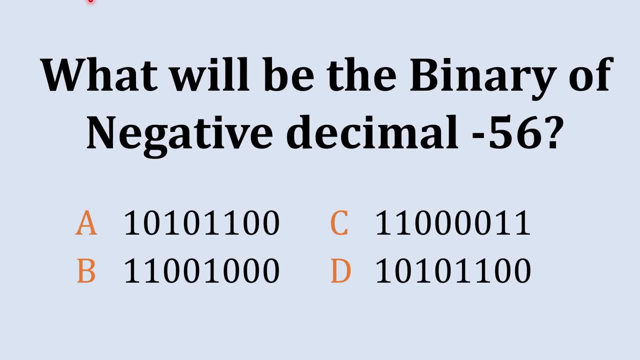 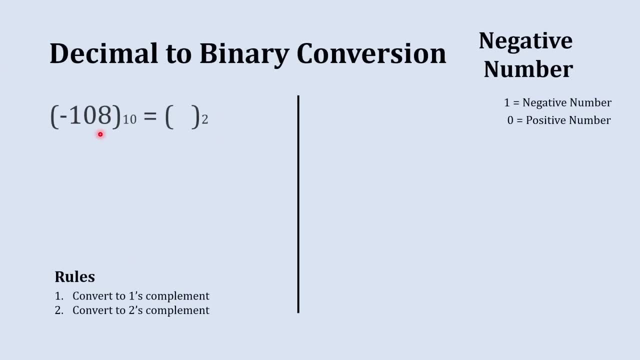 And your options are this: Pause the video, calculate it and post the answer in comment section below, And then we'll verify that how many of you gives the correct answer. Now let's jump for the next example, And here, our next example is 108.. 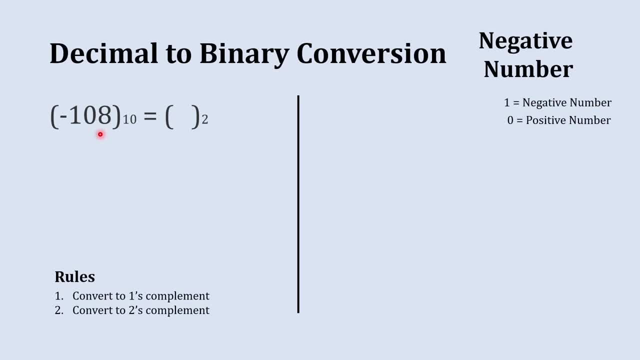 So we supposed to convert minus 108 into binary. So first we'll write 2 raise to 0.. 2 raise to 1.. 2 raise to 2.. So 1,, 2,, 4,, 8,, 16,, 32 and 64 are decimal equivalent. 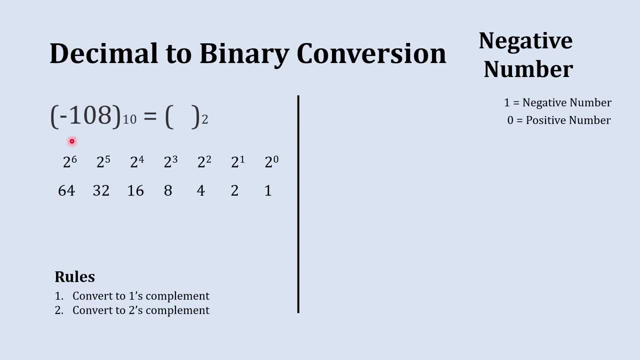 And now we supposed to add the numbers, which will gives us the total as 108. So first we'll take 64, as this 64 is less than 108. So we'll take 64, and then there is 32.. So if we add 32 into 64, it becomes 96.. 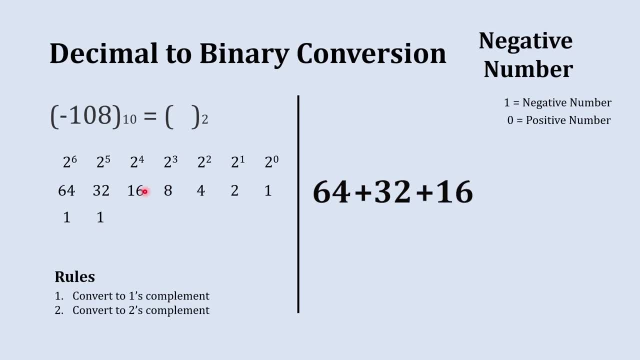 Yes, so we'll add this 32.. Now, if we add 16 into this, it will become 112.. So we'll skip this 16 and then we'll jump to next. Now we'll add 8.. So if we add 8, it will become 104.. 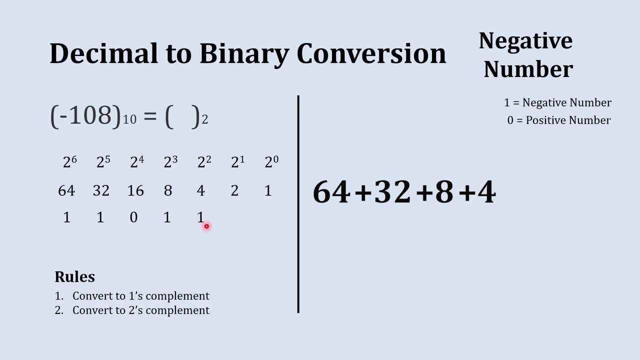 So we'll add 8.. Now we'll add 4.. So when we add 4 into 104, it will become 108. So we got 108. So now we do not supposed to add this 2 and 1.. 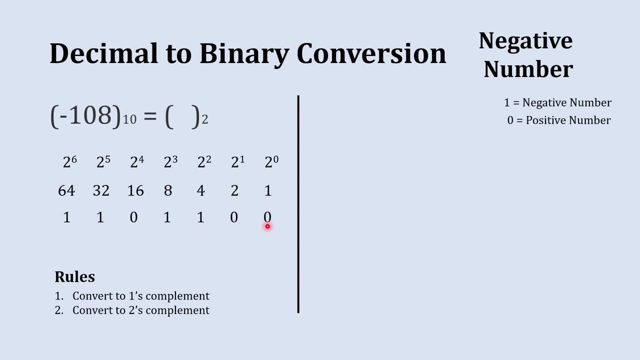 So this 110, 1100 is the binary equivalent to positive 108.. Now it's time to convert it into negative, And for that we have clear 2 rules. So first we'll write this number into 8 bit number. 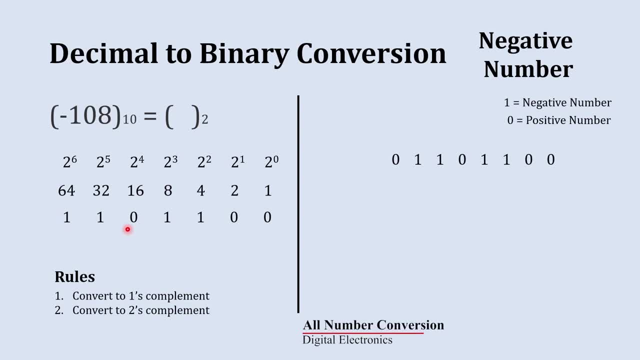 So this is the 8 bit representation. This number is already of 7 bit, So we supposed to add only 10 to convert it into 8 bit. Now we'll take 1's complement of this number. So wherever there is 0, we'll write 1, and wherever there is 1, we'll write 0.. 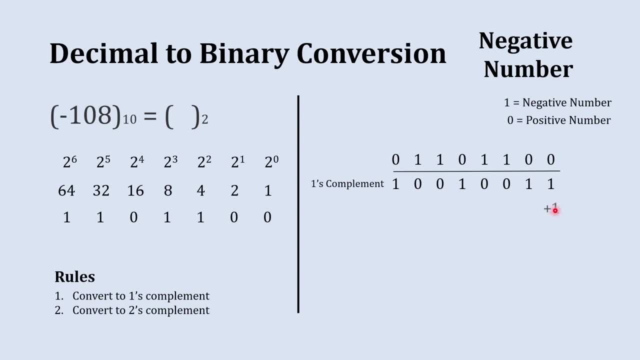 And now it's time to take 2's complement of this number. So in order to get 2's complement, we supposed to add plus 1.. So 1 plus 1, 0 and there is 1, carry. Now again 1 plus 1, the sum is 0 and 1, carry. 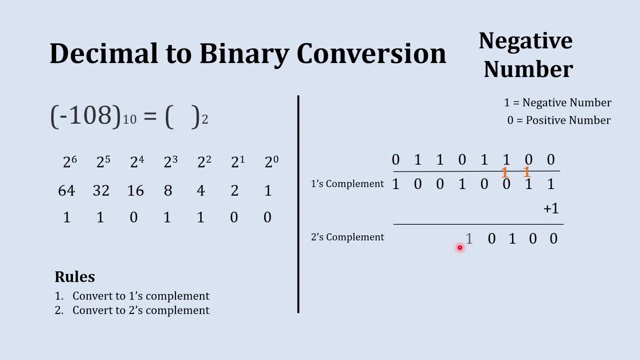 Now 1 plus 0, 1, 0, as it is 1, 0, 0 and 1.. So now this number is the binary equivalent to minus 108.. And we can write this thing in this manner: 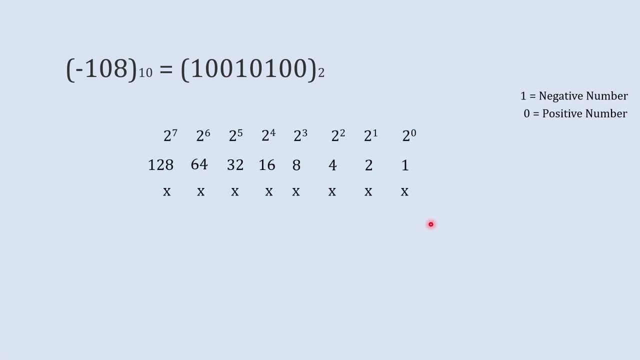 So we'll use the same previous method. We'll multiply this binary numbers with this decimal number And the most significant bit will keep it as minus. So minus 1 into 128 gives us minus 128.. Plus 64 into 0 gives us 0..